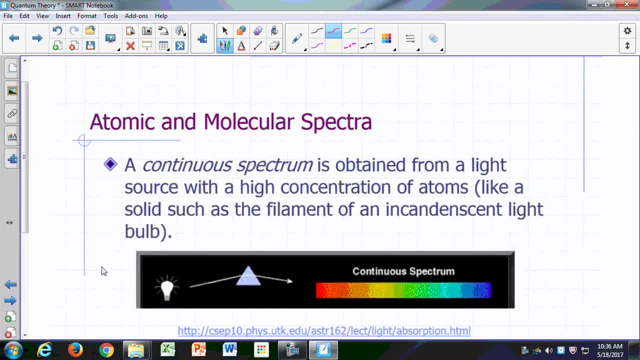 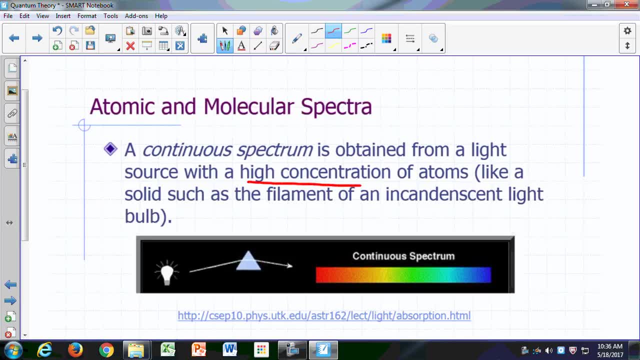 So let's take a look at a typical observation you might make. If your light source, the sample of matter that produces the light, has a high concentration of atoms, that means you've got a lot of atoms crowded in a very small space. okay. 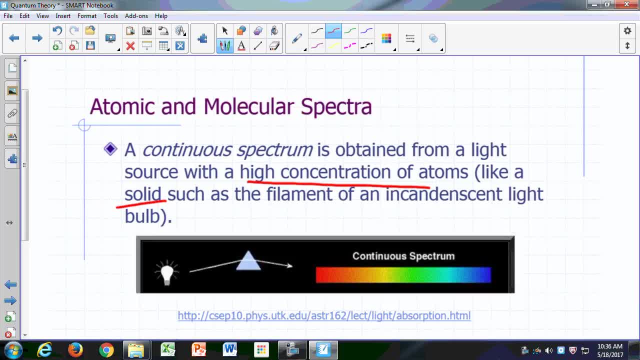 So, for example, in a solid the atoms are as close as possible to each other. So an example That would be like the filament of a light bulb. okay, So you run electricity the way it produces light. okay, And if you were to split that light into its component colors? what you typically see, if there's a high concentration of atoms from the light source, is what's known as a continuous spectrum. 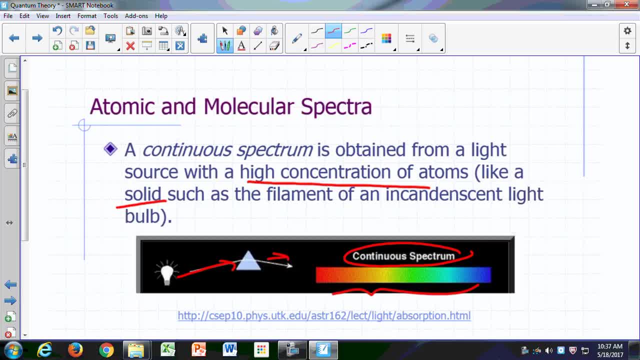 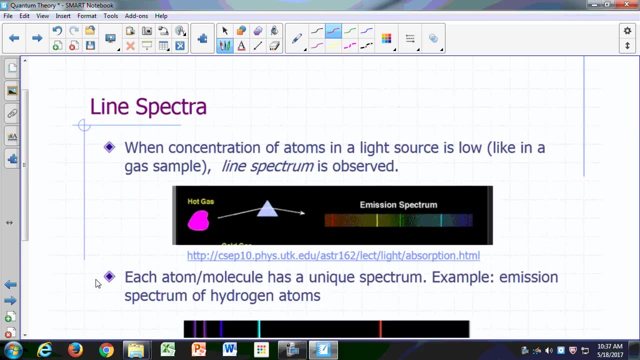 Continuous in the sense that you have a continuous band of colors, just like a rainbow, and you get to appreciate a little better exactly why we call it continuous if you look at what happens. So if your light source has a low concentration of atoms, so if the concentration of atoms in your light source is low, for example, if you have a gas sample right here, so you have a hot gas produces light, and you were to examine the light that's produced by the hot gas, so separate it into its component wavelengths, you can see you get what's called a line spectrum. 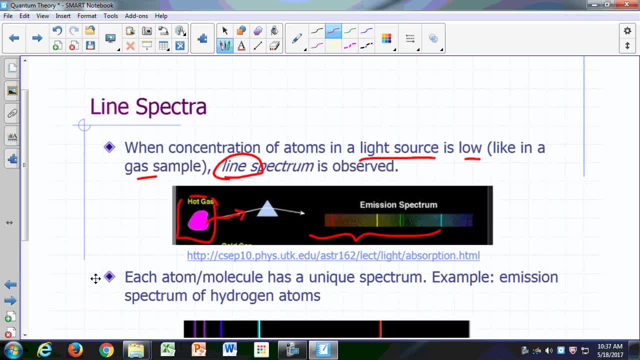 So this is a line spectrum. So this particular emission spectrum from a source that has a low concentration of atoms is a line spectrum. You can see it's mostly dark areas with very bright lines, a few bright lines in between. okay, Now this is called the emission spectrum, okay, or the line spectrum of the atoms that are producing the light in your hot sample of gas. 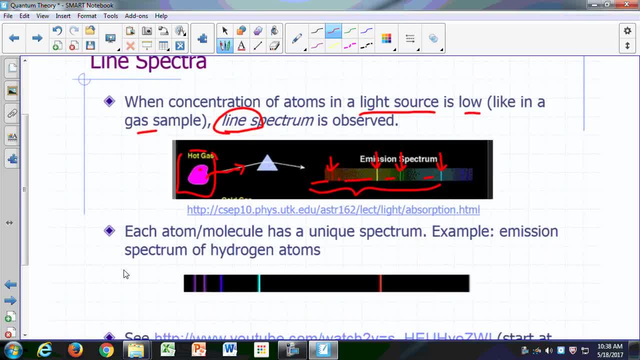 Now, each particular atom or molecule has a unique spectrum. So, for example, if your sample only contains hydrogen atoms- In other words, the only atoms producing light from your sample are hydrogen atoms, and the concentration is low- This is typically what you'll find. 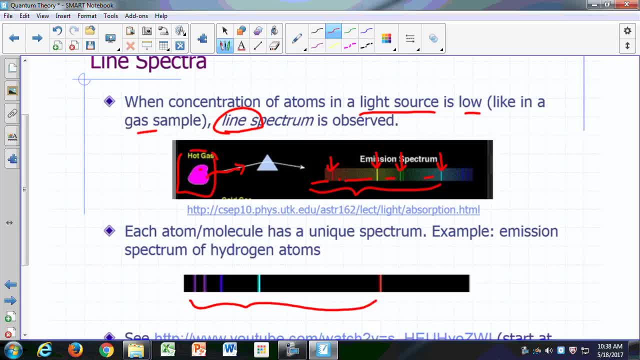 This is a characteristic of hydrogen atoms. So, in a way, the light being produced by atoms is an identifying characteristic of the atoms. It's their ID number. you might say It's their fingerprint. okay, Each atom has a different spectrum. characteristic spectrum.